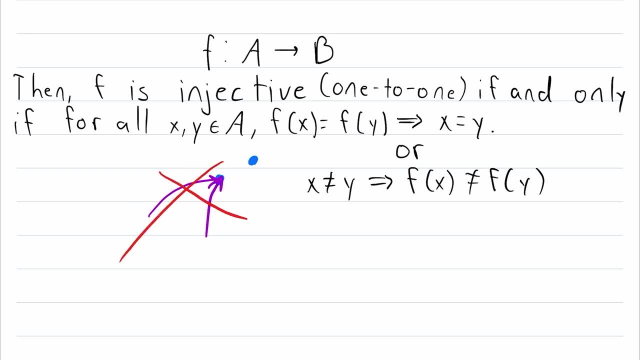 be mapped to more than once. So something like this would not be allowed in an injective function. And notice that there are three terms here that mean the same thing: An injective function is sometimes called an injection, which is sometimes called a one-to-one function, Another way to think. 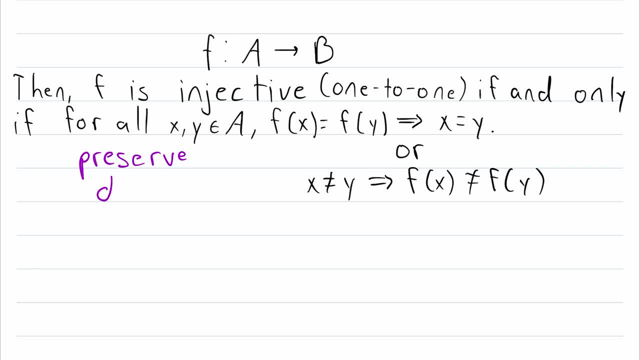 of injective functions is that they preserve distinctness. I think this is a great idea to think about it. If two elements of the domain are distinct, then their images after getting put through the function must also be distinct. That's what makes a function injective. Let's 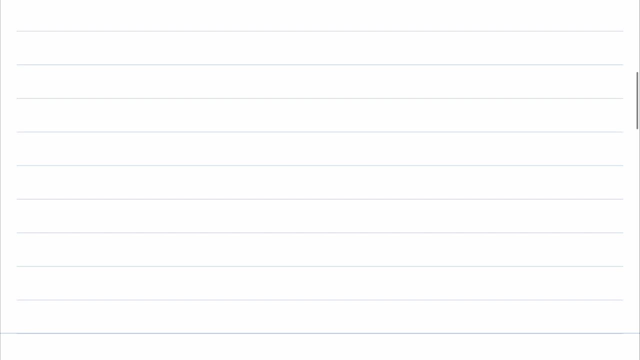 quickly take a more detailed look at a diagram to get a better idea of injections. Let's say, this set is a the domain and this set b over here is the codomain. We'll put a few elements in our codomain and we'll put a few elements in our domain. 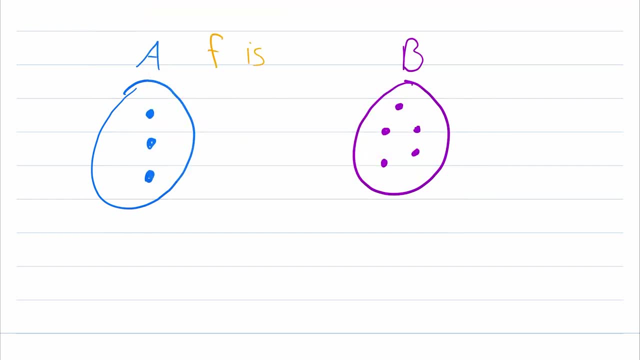 So we'll put a function to be an injection and we'll say that f is an injection. It's an injective function. Distinct elements of the domain have to map to distinct elements of the codomain And that's why injective functions are sometimes called one-to-one functions. One element of the domain. 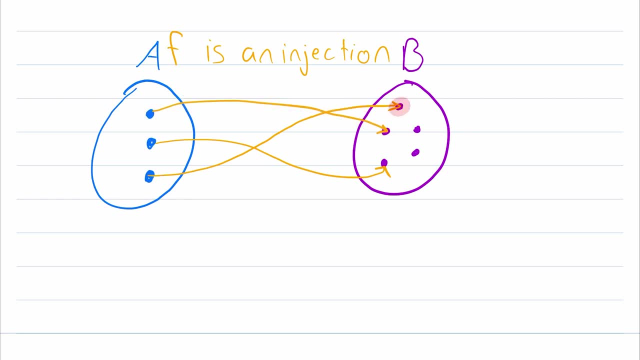 maps to one element of the range and every element in the range gets mapped to exactly once. Notice in this case that the range is this and the set of elements here, So not every element in the codomain is getting mapped to, and that's totally fine for an injective function, But it's not fine for another type of function. 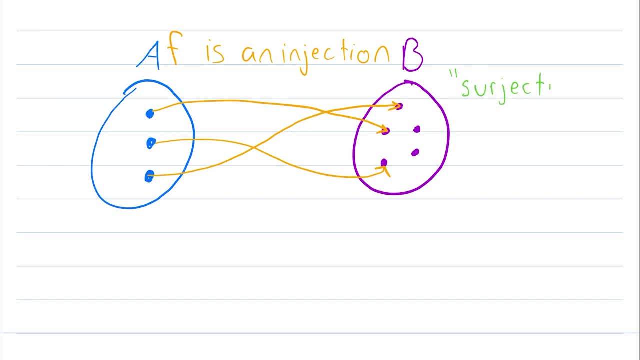 called a surjection, And we'll talk more about those in another lesson. Just to show you what a non-example would look like if this element of the domain mapped to say this element of the codomain. this is no longer an injection, Because we've got two distinct elements of 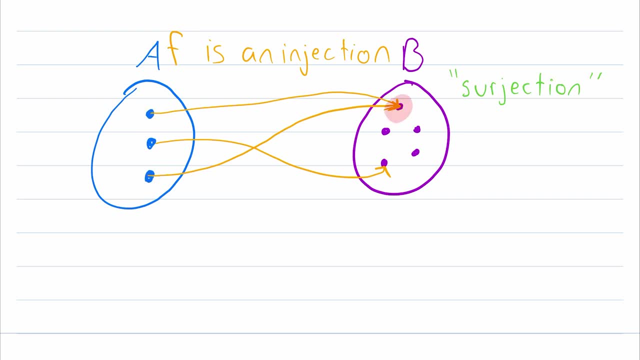 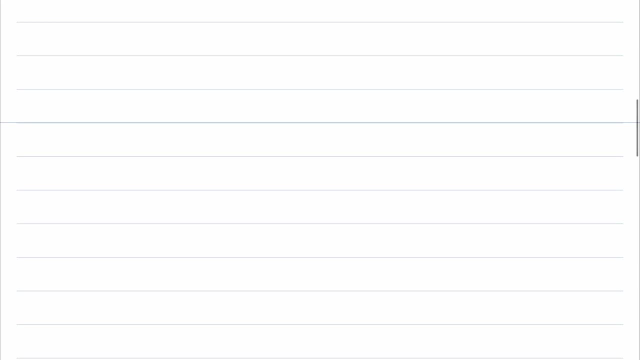 the domain mapping to the same element of the codomain, So that would not be an injection. Now let's take a quick look at how we might prove a more concrete example of an injection. Let's say our function f maps the real numbers to the real numbers and it's defined like this: f. 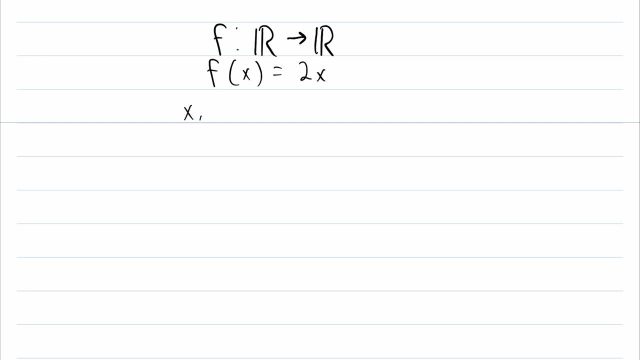 is equal to 2x, Then we'll take two elements- x, y- from the domain. Suppose that f is equal to f, then, by definition of the function, 2x is equal to 2y. Divide both sides by 2, x is equal to y. 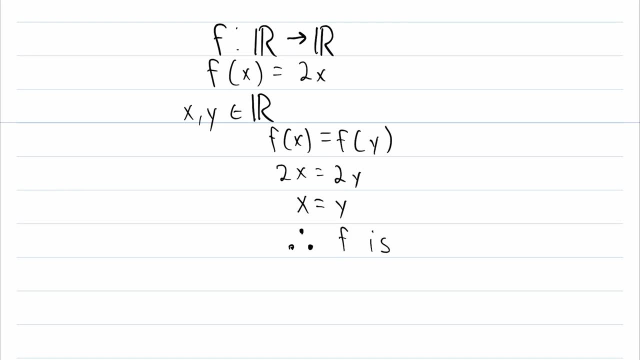 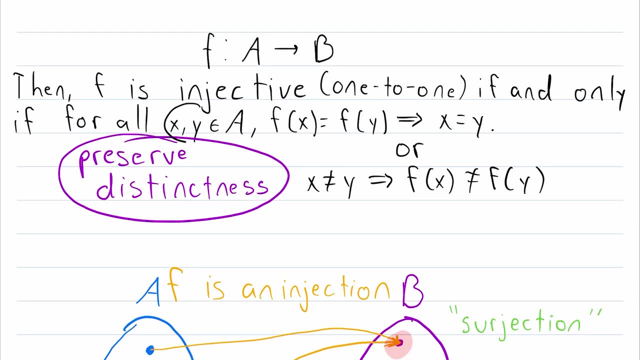 Therefore, by definition, f is injective. So this is a super straightforward proof. just uses the definition we went over above For any elements x, y of the domain. if f of x equals f of y, implies that x equals y. then the function is injective. And in the example we just looked at, since this 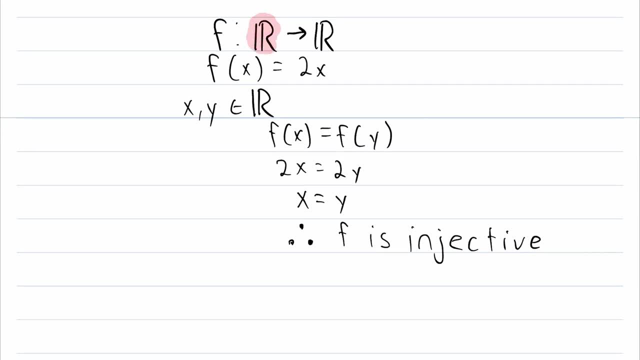 function f is differentiable on its entire domain. we could also prove that f is injective using calculus, because the derivative of f is equal to two. If the derivative of a function is always positive or always negative, it can easily be shown that it is injective using that contra. 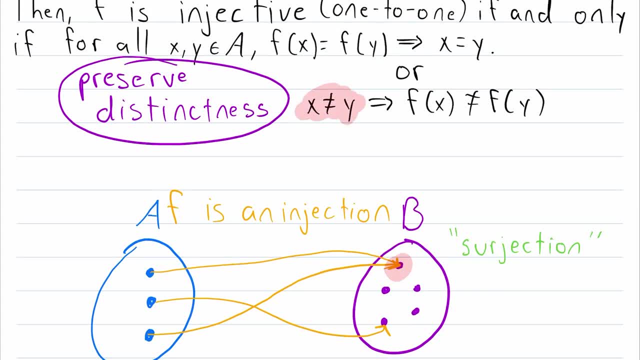 positive we talked about earlier. The fact that x not equaling y implies that f of x is not equal to f of y, And if it's not clear to you how that would work, don't worry too much about it, but take some time to think about it. But most 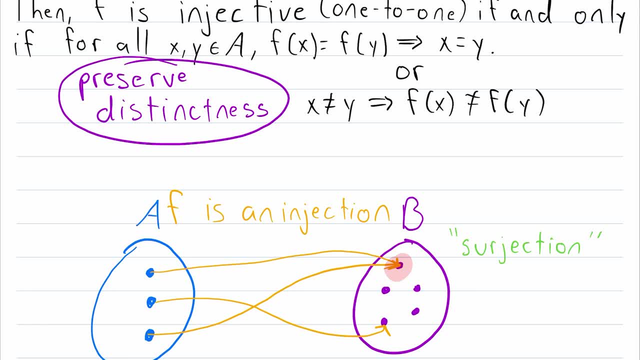 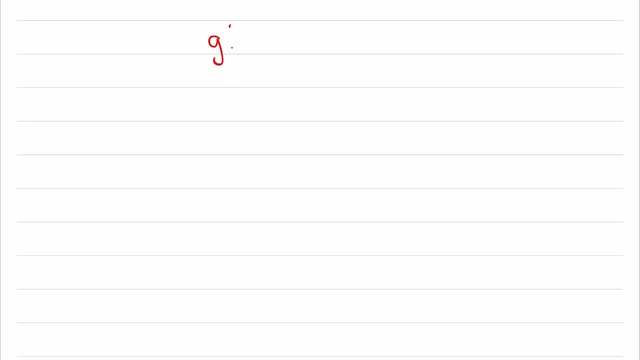 importantly, what I want you to get for this lesson is what an injective function is. And quickly, to make sure you understand, let's take a look at a more concrete non-example. Let's say we've got a function g that again maps the real numbers to the real numbers, and g is defined like this: g of x. 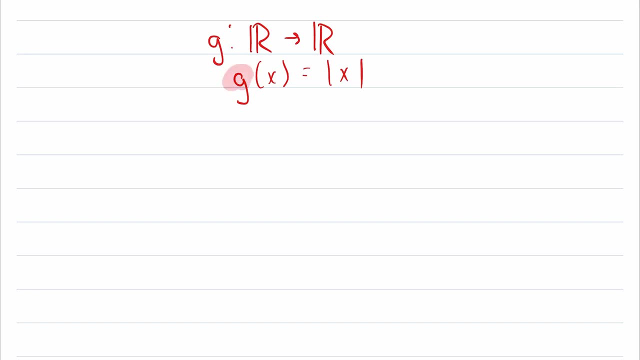 equals f of x. g equals the absolute value of x. g is not an injective function And we can prove this by counterexample showing that the contra positive doesn't hold. We take two distinct elements from the domain- negative 3 is not equal to positive 3, and then show that their images are equal. g of. 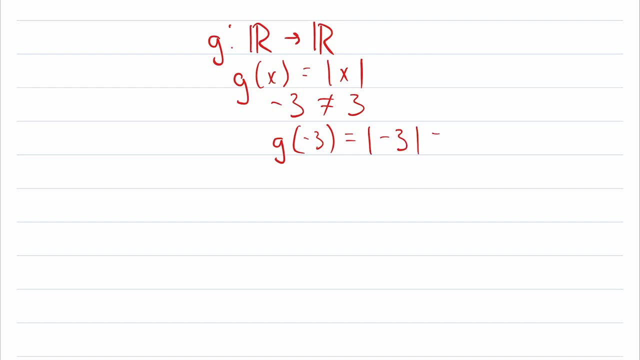 negative 3 is equal to the absolute value of negative. 3 is equal to positive 3.. g of positive 3 is equal to the absolute value of positive 3.. Therefore, g of negative 3 is equal to g of positive 3.. Therefore, g is not injective.